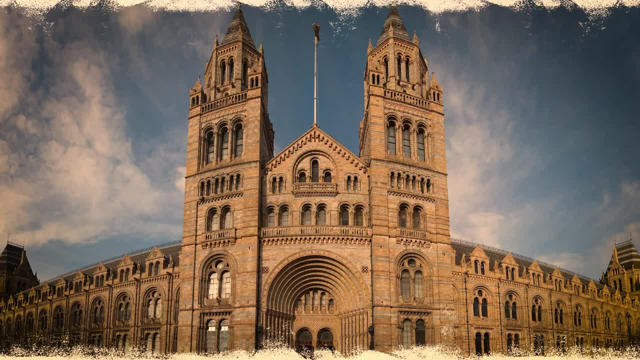 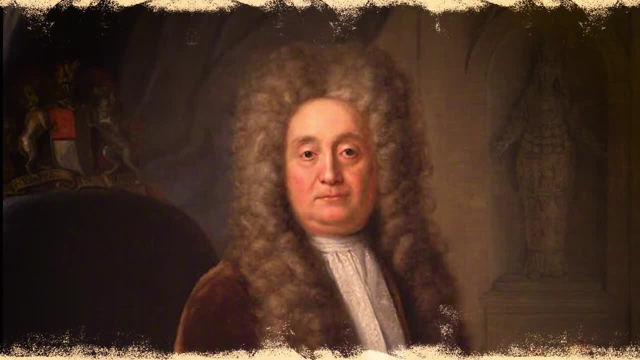 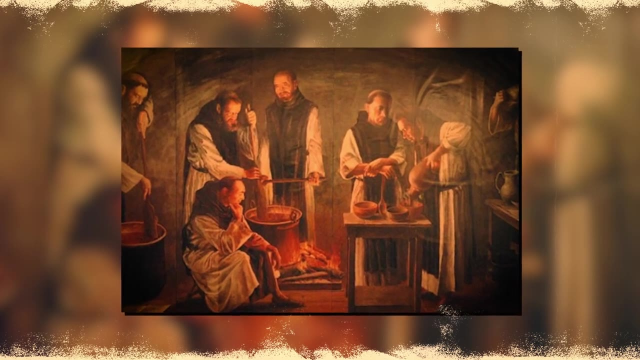 century that a breakthrough occurred. According to the Natural History Museum in Britain, that credit goes to Sir Hans Sloane, an Irish botanist. The story goes that Sloane spent some time in Jamaica in the early 1700s where the local people gave him cacao to drink. He found 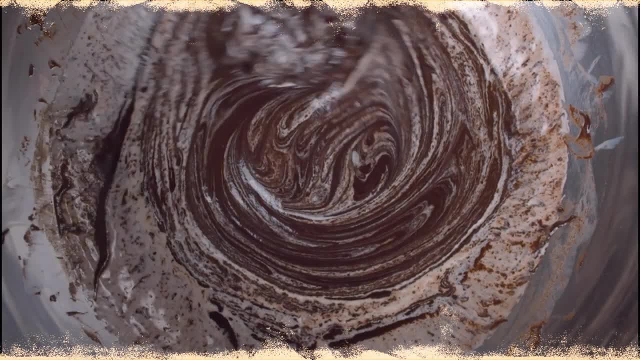 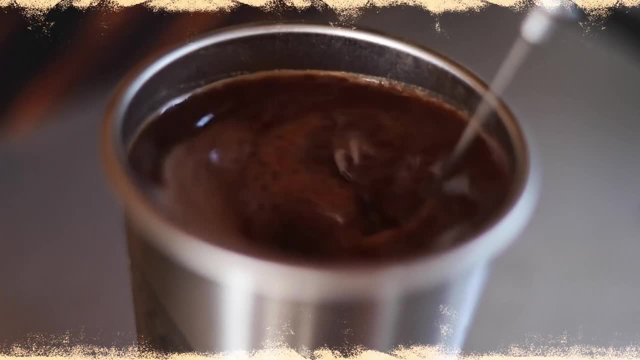 it nauseous, but by mixing it with milk made it more palatable, according to the museum. When he then returned to England, Sloane brought the milk and cacao mixture with him, and for many years his recipe was sold as medicine. In the early 1800s Sloane was given the cacao to drink, but he didn't. 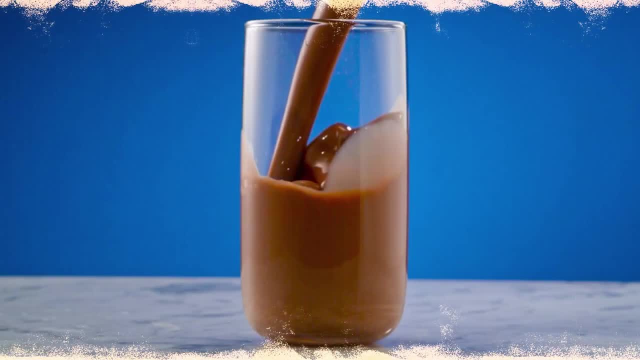 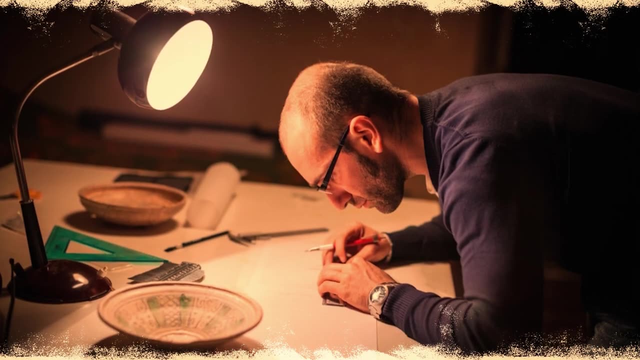 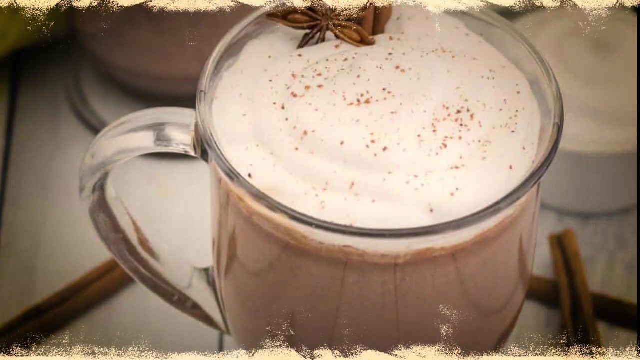 get the credit for inventing the cacao. According to many historians, the Jamaicans were brewing a hot beverage from shavings of freshly harvested cacao boiled with milk and cinnamon for as far back as 1494, and more than likely even further than that, Considering chocolate had 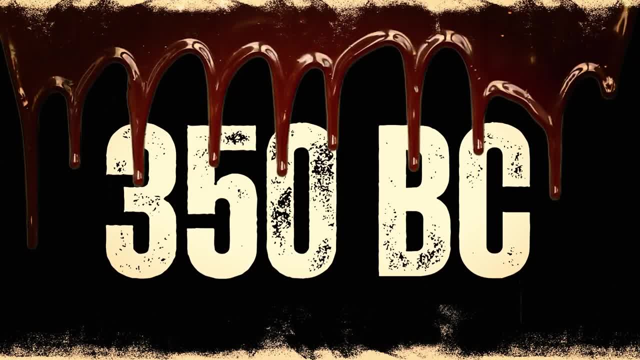 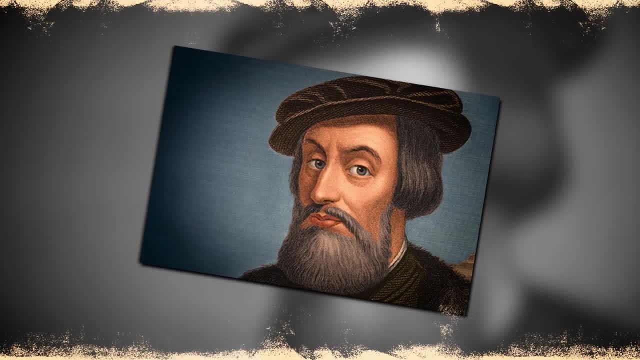 been known to humans as far back as 350 BC. it's much more likely that Jamaica had some form of chocolate milk already, and then Sloane is credited with the invention because he was the one that spread it on an international scale when he returned to the UK, unlike Spain, 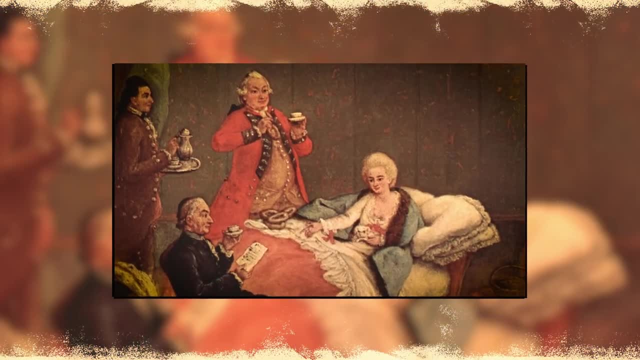 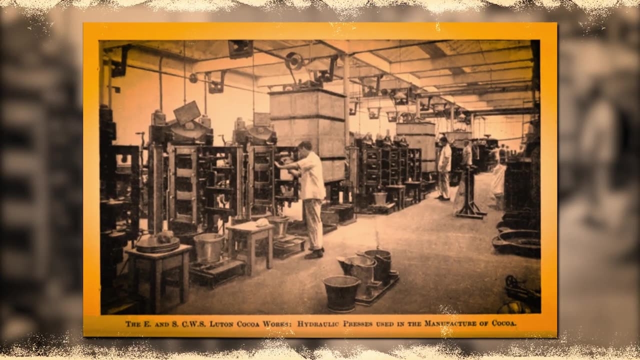 who wanted to keep it a secret for monetary purposes. But as the years passed, chocolate milk evolved and made its way across borders. In the 18th century, the industrial revolution changed the production of chocolate. Innovations in processing techniques made it possible to produce chocolate on a larger scale by creating a powdered form, bringing its cost down and making it accessible to a wider audience. Marry that with 19th century significant advancements in the dairy industry leading to the mass production of milk, and you've got a recipe. 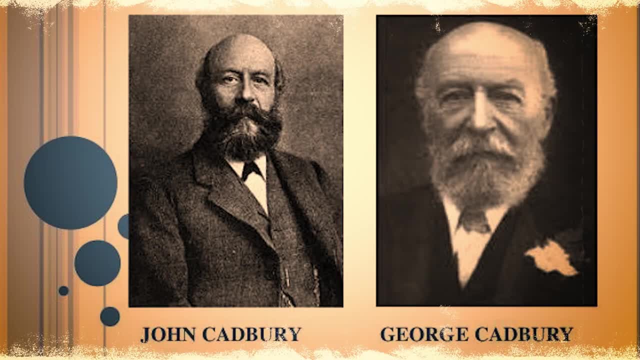 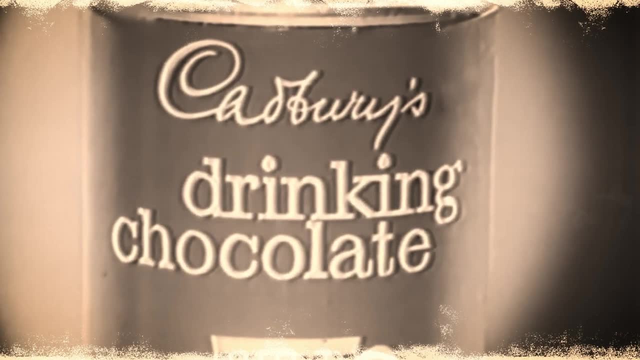 for chocolate milk popularity. Then, in the 1820s, the Cadbury brothers purchased the chocolate milk recipe from Sloane and used it to create a lucrative drinking chocolate business, still in business to this day. This development saw the availability of affordable chocolate. 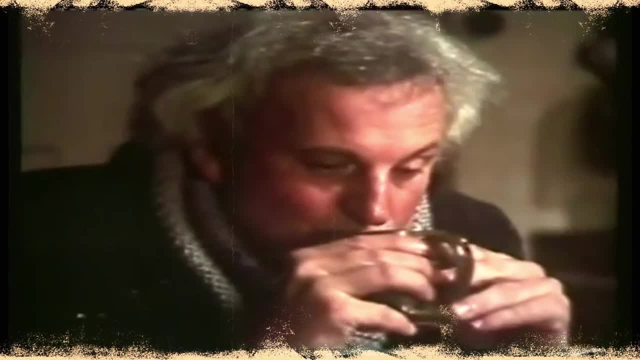 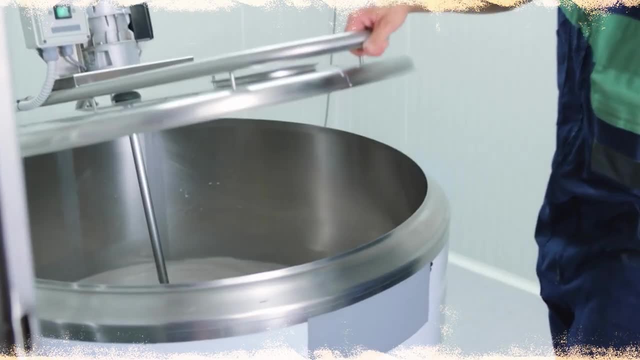 not as a medicine any longer but as a pleasure product, and paved the way for the widespread popularity of chocolate milk among the general public In the early 20th century. pasteurization techniques improved milk's safety and shelf life, making it an easier-to-acquire ingredient for chocolate milk. 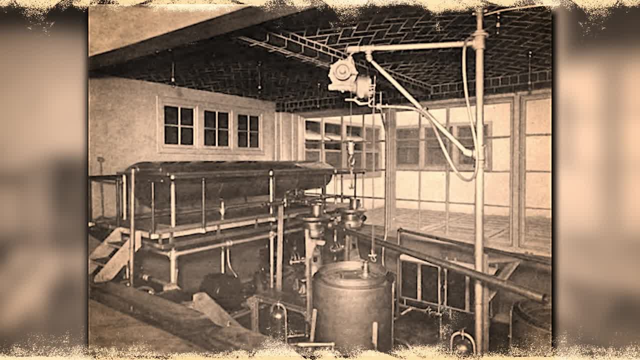 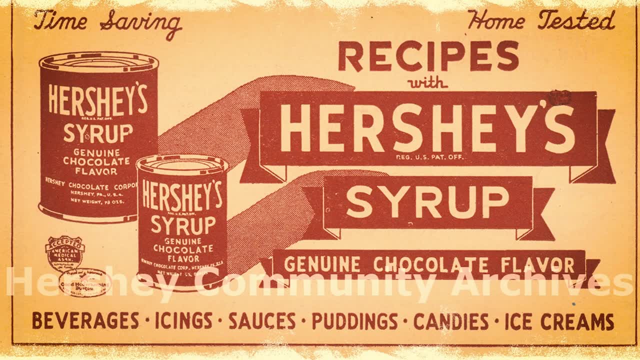 In the United States. the innovative use of automated milk processing and bottling machines further contributed to the rise of chocolate milk as a beloved beverage. and in 1926, we saw Hershey release the first chocolate syrup to be used for chocolate milk, And then, around 20 years later,